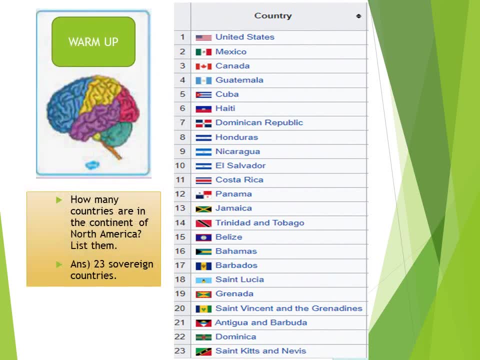 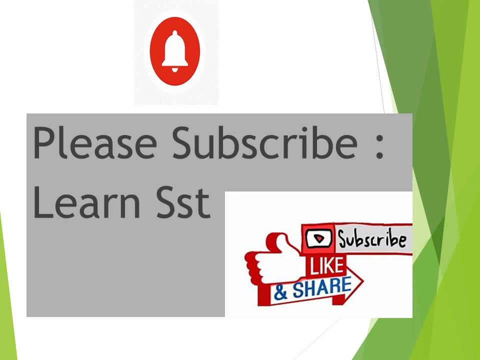 Here we have the warm-up exercise from our textbook. How many countries are in the continent of North America? List them. So there are 23 sovereign countries. The list you can see over here. So, viewers, before I proceed further with my video, just a humble request to please subscribe to my channel if you haven't subscribed. 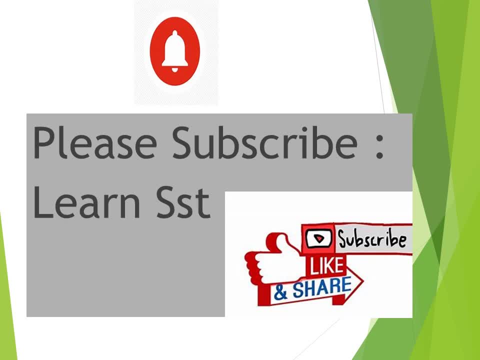 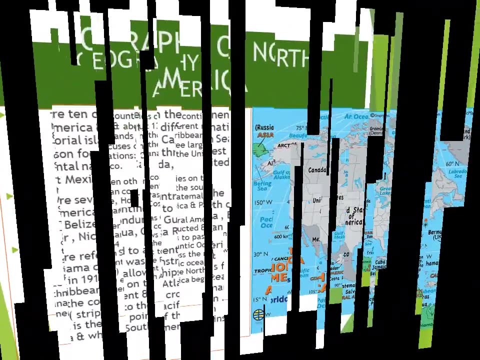 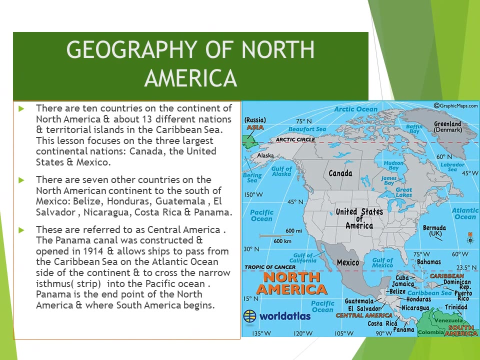 And please subscribe to my channel. if you haven't subscribed, Please press the bell icon for the notification of my latest videos. So here we have, the geography of North America. What you can see over here is the map of North America. When you look at the map of North America and you read the information provided, it gives you a better picture. 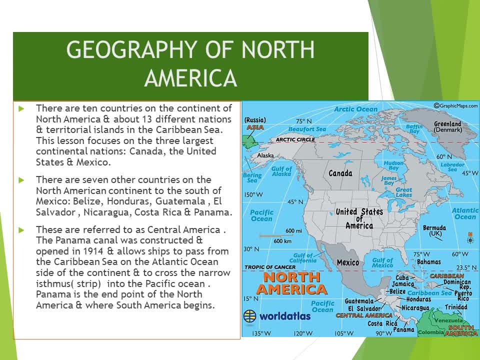 There are 10 countries on the continent of North America And about 13 different nations and territorial islands in the Caribbean Sea. This lesson focuses on the three largest continental nations, That is, Canada, United States of America and Mexico. So what you can see over here in the map, you can see in the northern region, Canada. 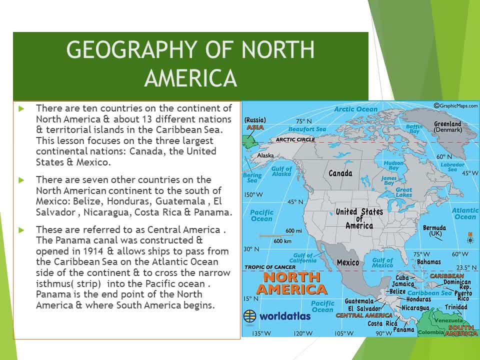 Then in the central part you can see the United States of America, And then you have Mexico. So this is what we have: the North America being divided into three main territories. There are seven other countries on the North American continent to the south of Mexico. 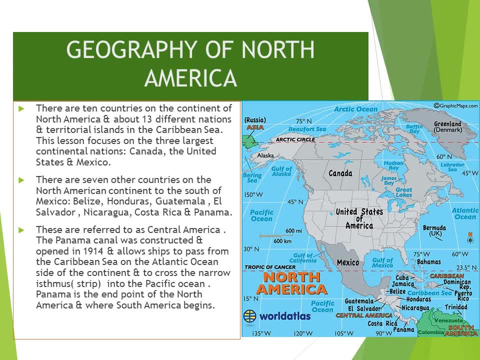 So these are the names of the countries: Belize, Honduras, Guatemala, El Salvador, Nicaragua, Costa Rica and Panama. These are referred to as Central America. The Panama Canal was constructed and opened in 1914 and allows ships to pass from the Caribbean Sea onto the Atlantic Ocean side of the continent and to cross the narrow isthmus into the Pacific Ocean. 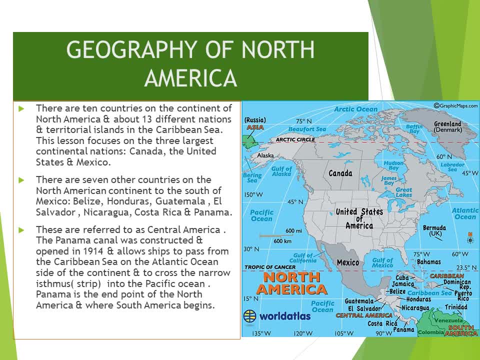 Panama is the end point of North America and where South America begins. So you can have a look over here in the map viewers. Just below Mexico you can see these Central American countries, which is very much clearly given over here, And then you can see at the edge, before the South American continent begins, we can see the Panama. 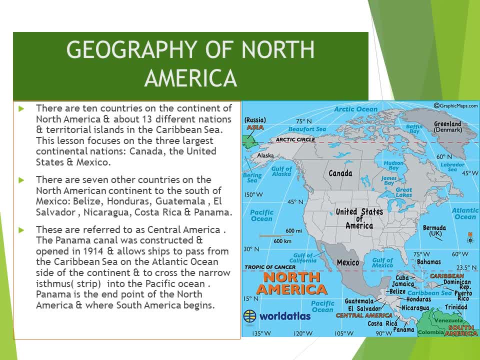 So we have a Panama Canal over here and this canal is helpful in connecting the two seas. One is the Caribbean Sea onto the Atlantic Ocean And then the other is the Caribbean Sea onto the Atlantic Ocean And then the Caribbean Sea onto the Atlantic Ocean. 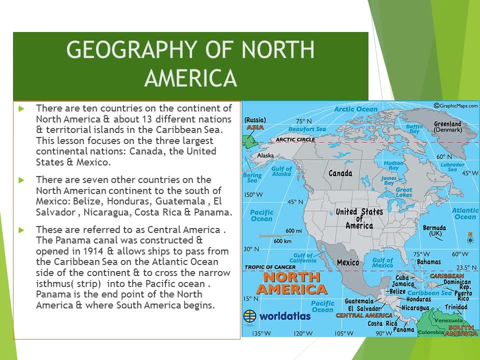